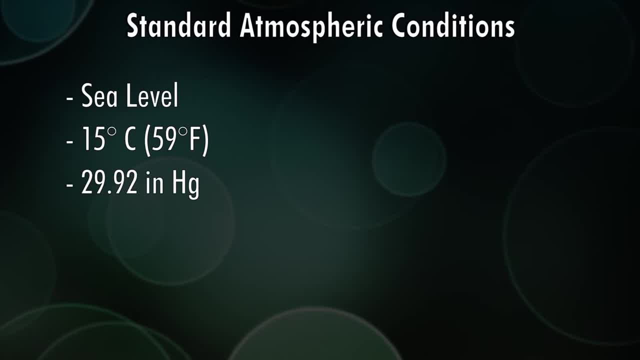 As you might imagine, we don't have those conditions happening all the time, And that's why we have performance charts so that we can interpolate and calculate our performance for our particular day at our particular airport, in our particular airplane. Things that affect your performance negatively are high humidity, high temperature and high altitude. 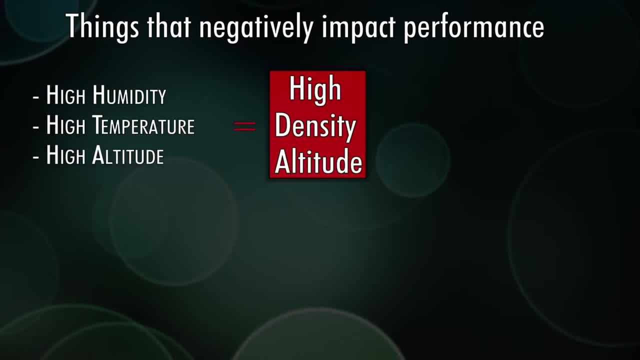 You combine all those, you get a high density altitude. Now, if you remember, a density altitude is pressure altitude corrected for non-standard temperature. In plain English, density altitude is the equivalent altitude that the airplane thinks it is at and it performs accordingly. 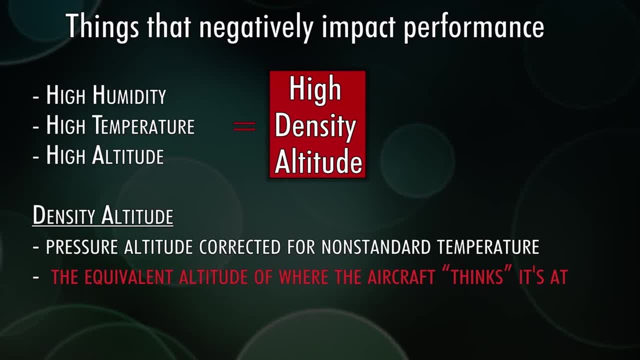 In other words, when you have a high density altitude, the air is thin, so you have less lift, your engine produces less power and your propeller produces less thrust, And so all those things combined, you have a high density altitude. 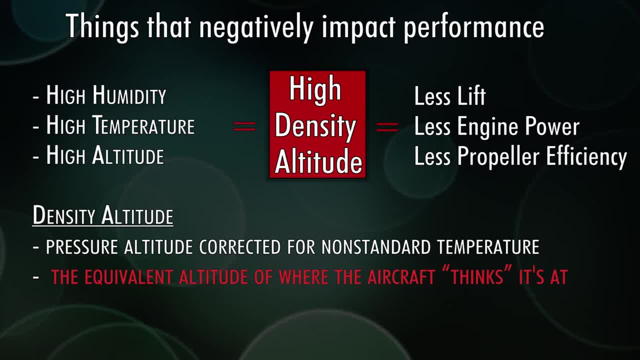 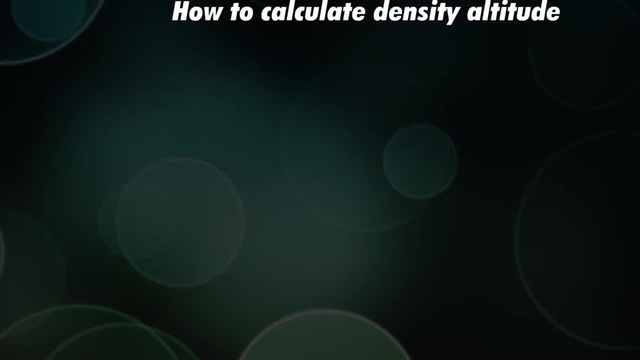 The airplane thinks it's super high when in reality it really isn't. It feels like that because the air is a lot thinner due to all those factors. Now then, how do we find this pesky density altitude? We take our elevation. we correct that for non-standard pressure. 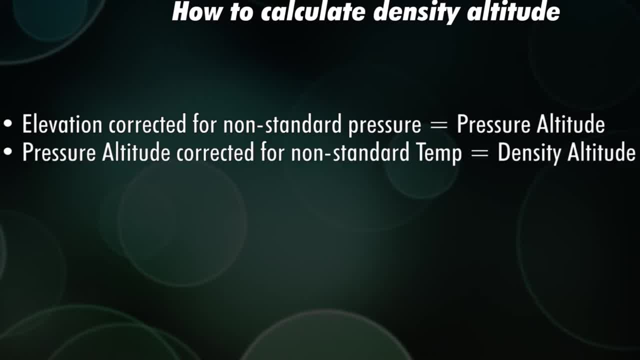 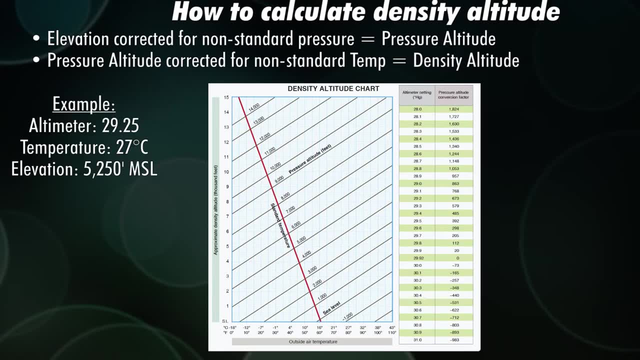 That'll give us our pressure altitude. We take the pressure altitude, correct it for non-standard temperature and you get density altitude. And, believe it or not, there's a chart for that. Here's an example we'll work through. We'll say our altimeter is 2925, 27 degrees Celsius and the elevation is 5250.. 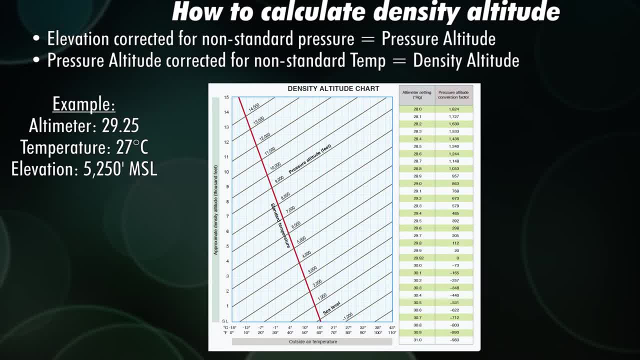 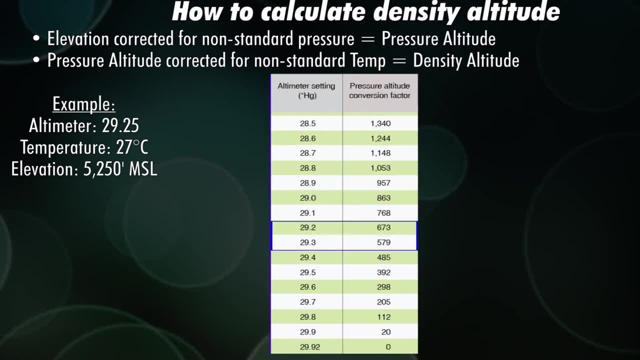 So the way this chart works on the right hand side you can correct for your non-standard altimeter. In other words, if it's not 2992 outside, you need to correct for non-standard pressure. Our altimeter is right between 29.2 and 29.3.. 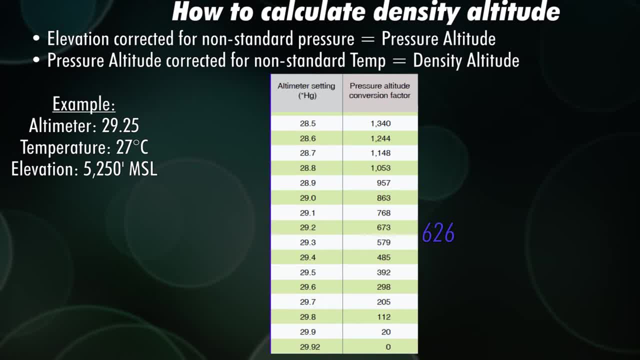 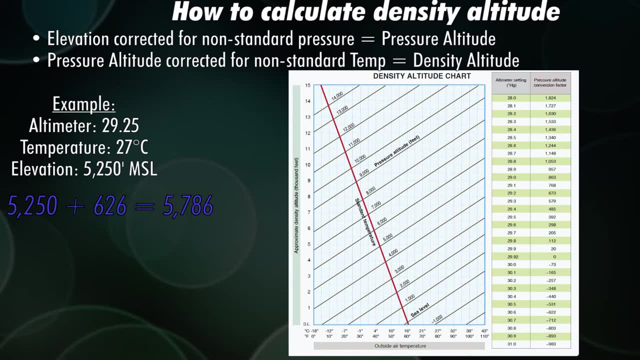 So if we work out the little interpolation there, that's 626 feet that you have to add to your elevation to get your pressure altitude. Now if we look at the left hand side of the chart, you can come in with that pressure altitude of 5876.. 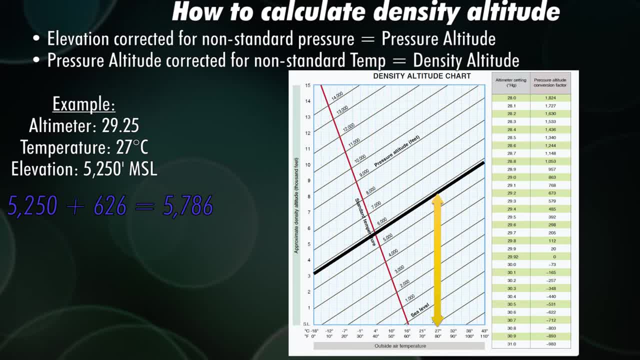 From the bottom you can follow the temperature line And then where they intersect. if you go all the way over to the left, it's going to give you your density altitude of 8500 feet. In other words, you are at an elevation of 5000 feet. 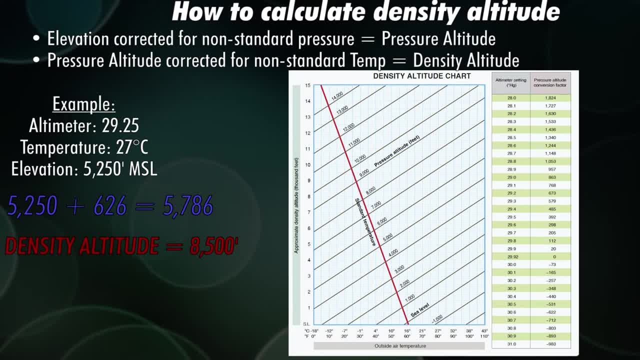 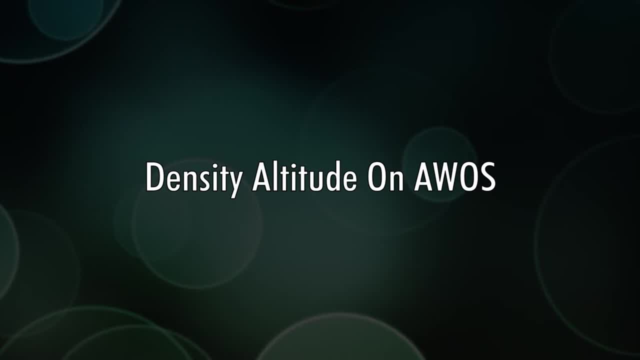 But your airplane, when it takes off, will feel like it's taking off. It's taking off from 8000 feet elevation. On a lot of the automated weather stations you'll hear density, altitude, like at this airport. Automated weather observation. 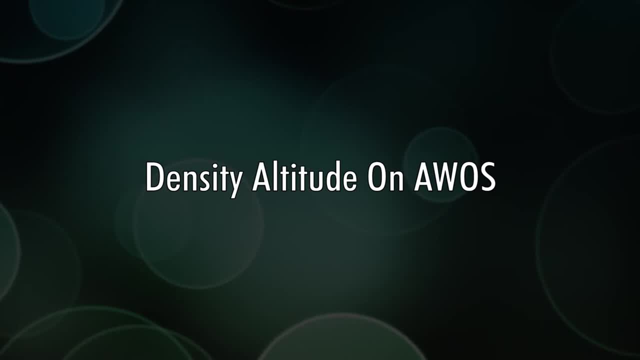 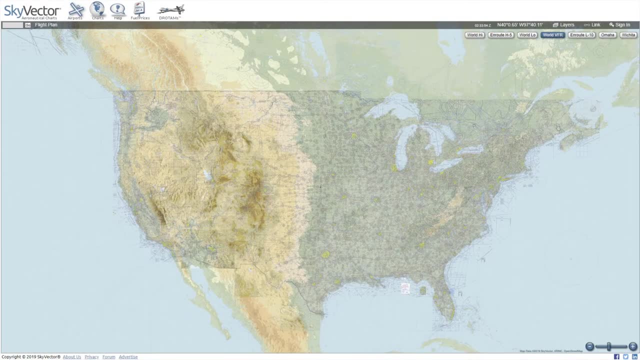 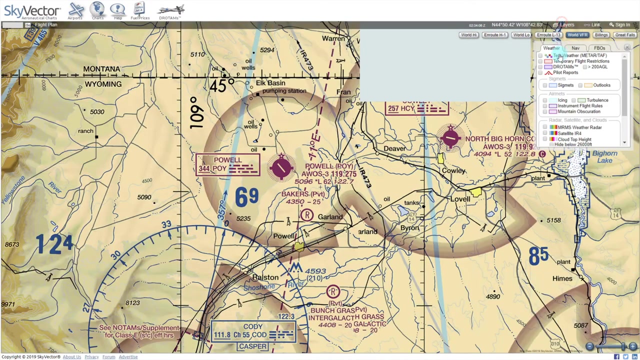 Altimeter 2998.. Remarks: Density altitude: 1300.. So now you know how to find density altitude. let's look at an actual airport with some weather to do our performance calculations. I'm going to go to SkyVector and zoom in to this lovely Papa Oscar Yankee airport. 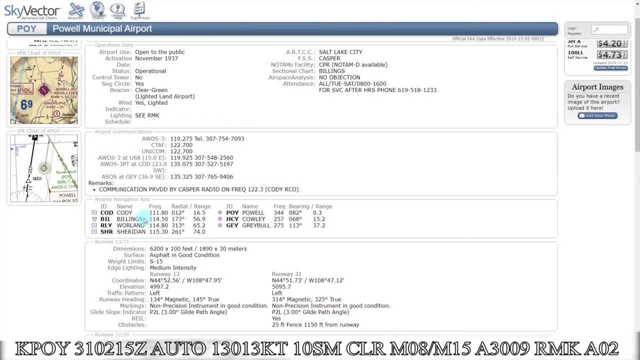 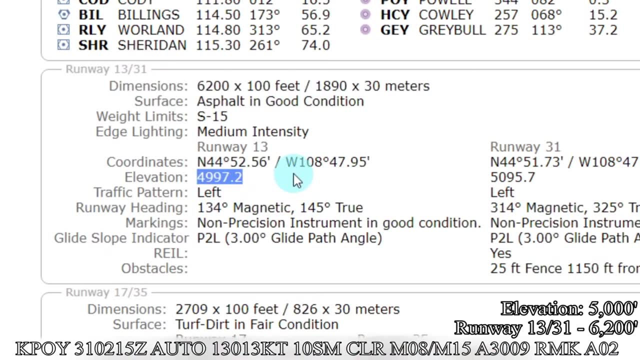 And here's the weather at that airport. Opening up the page, you see that it's got runway 1331 and it's 6000 feet long. The elevation is 5000 feet. The chart I'll be using in this example is from a Cessna 152.. 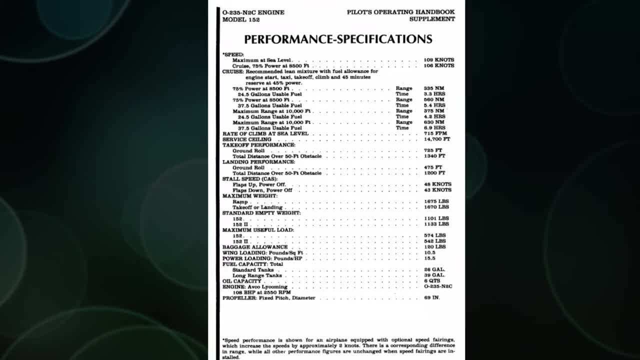 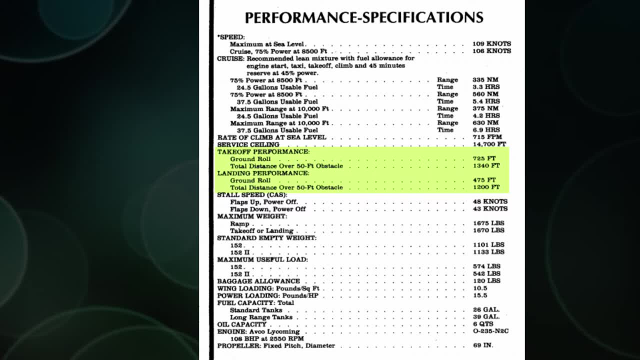 Keep in mind a couple of things. One of them is that some manufacturers do not provide really good takeoff data, like this example. You only get a couple numbers for takeoff and landing and you can't account for any other temperature and pressure differences. 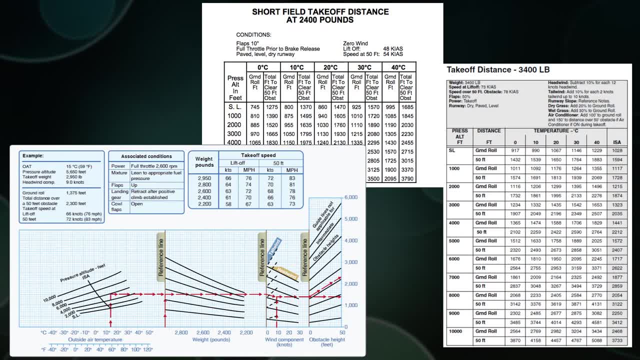 Another little note is that different manufacturers provide different temperatures. Different manufacturers provide different looking charts, and we'll go through a couple of them just so you're familiar with them. A really big emphasis on these performance charts is that you always want to read the terms and conditions. 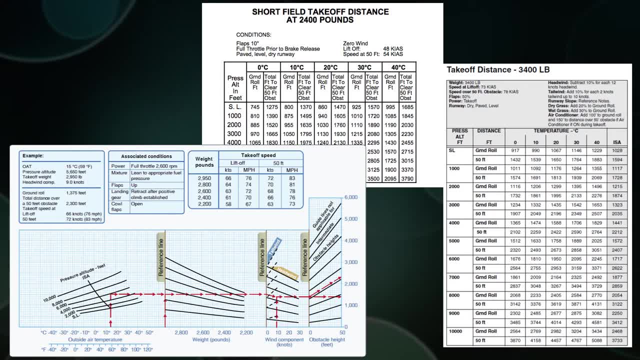 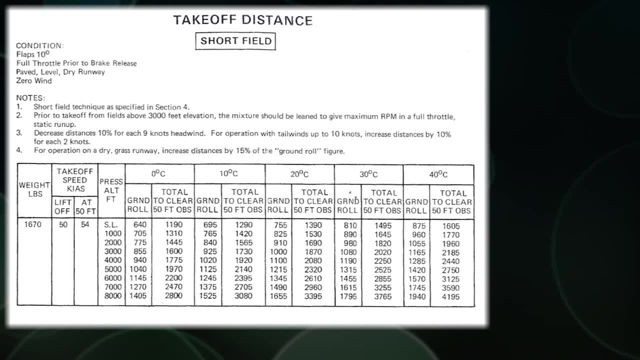 All the notes, all the conditions, all the stars and everything that's in the chart. Make sure you read all those little notes because it could come into play. For example, in our takeoff chart it says that you'll be using flaps 10.. 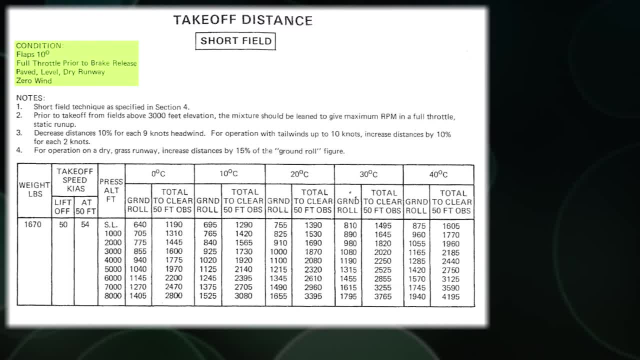 You'll have full power before you release the brakes and you're going to be on a paved runway with no wind. That's probably not going to be the case, And also one of the notes says that you'll be using a short field takeoff. 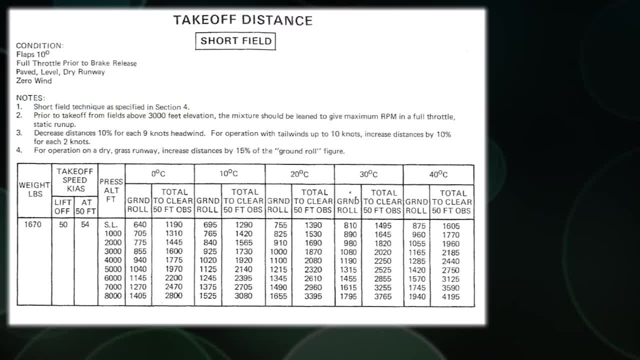 Chances are, that's not how you'll be taking off, So make sure you read everything there and get familiar with what the numbers say, Also in real life. add a bunch of distance to your numbers, just in case. Alrighty, then let's actually look at this little chart. 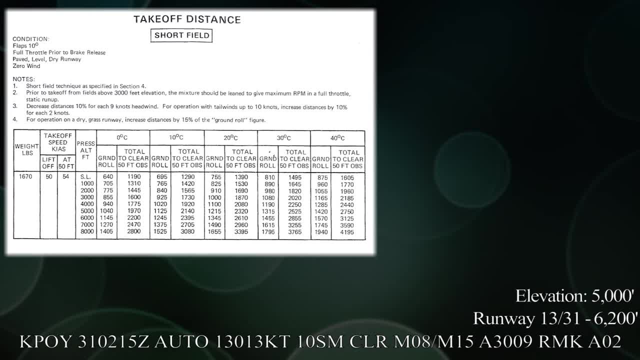 So we know our elevation is 5000 and if we look, our temperature is minus 8.. Our chart only goes down to 0 degrees And since we don't have anything negative, We'll just use 0.. This will be a quick example, so we won't do the pressure altitude conversion thing. 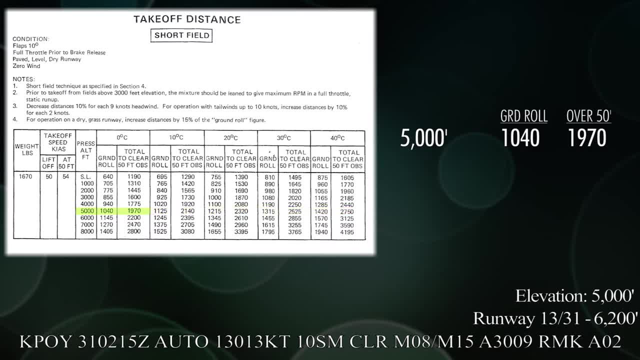 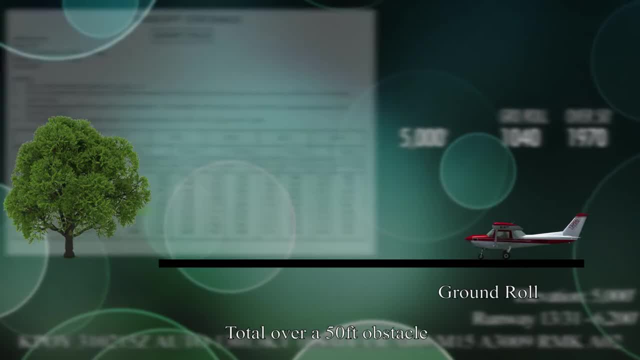 But we'll just look at the ground roll of 1040 and the total to clear a 50 foot obstacle of 1970.. Just as a review, the ground roll number is from when you apply power to when you get off the ground. 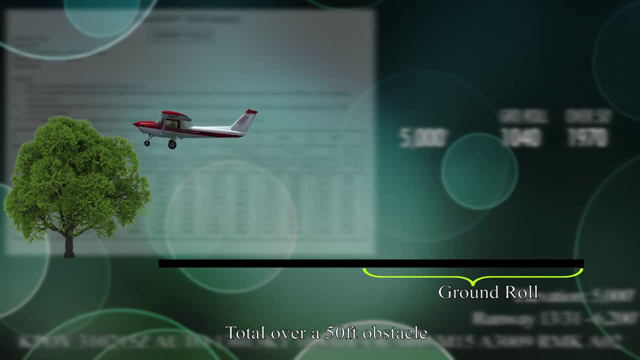 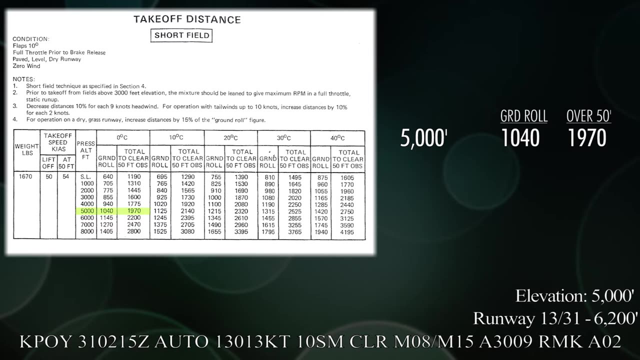 And the 50 foot obstacle number is from when you applied power until you took off and then climbed 50 feet. Okay, so our 5000 foot numbers are 1040 and 1970.. Now, if we read the notes like we should, 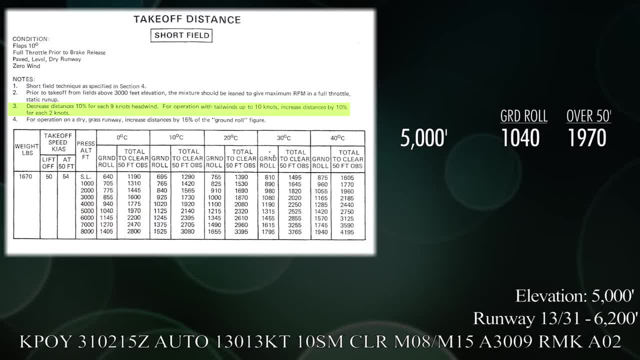 Number 3 says you should decrease your distances 10% for every 9 knots of headwind. So if we take 13 knots, that our wind is Divided by 9. You get 1.44.. You multiply that by 10%. 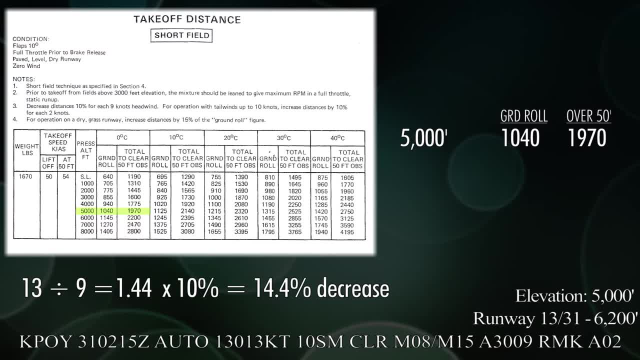 You get 14%, in other words 15% of a decrease in your takeoff distance. So we can subtract that from our ground roll number and the 50 foot obstacle And you get 884 and 1675.. Now those are the numbers you would put on a written test. 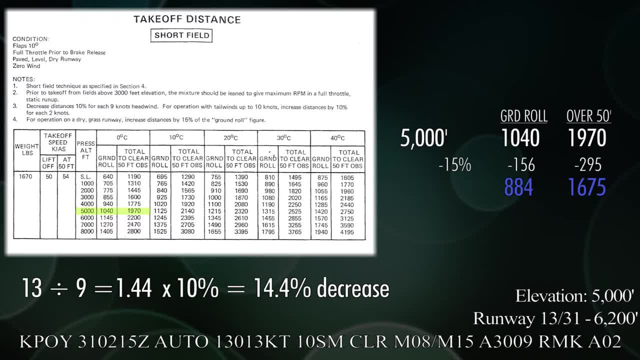 In real life I would probably shoot for about 1200 feet on the ground roll And let's say 22,, 2300 feet on the over 50 foot obstacle, Just to be on the safe side. That's simple enough, right. 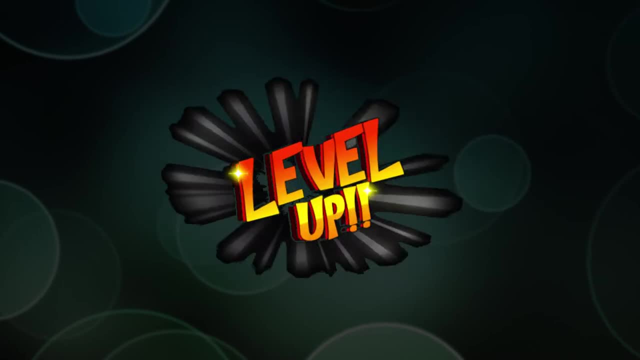 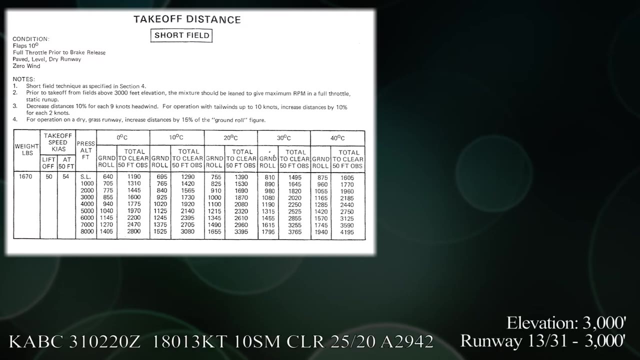 Let's level up and do a difficult example. Here are some new numbers for the new example. Here's your weather. We'll be at an elevation of 3000 feet. Our runway is still the same runway. We'll just make it 3000 feet for laughs and giggles. 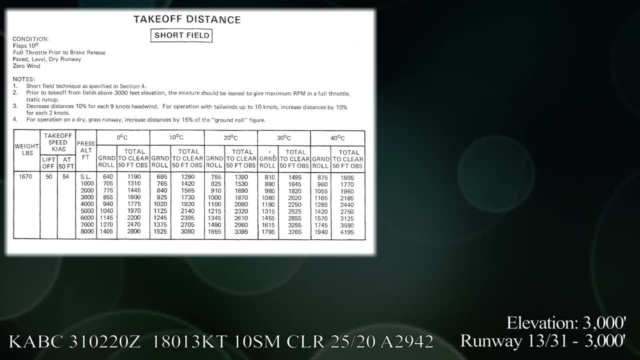 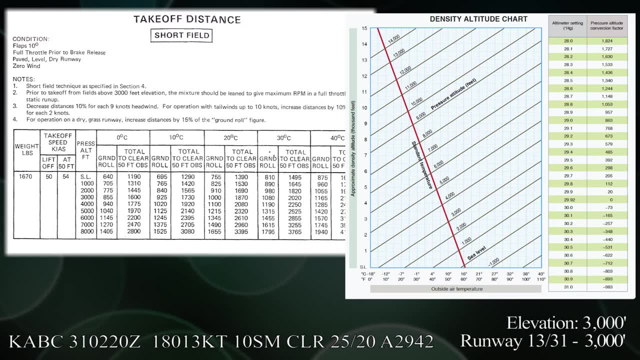 First of all, we need to figure out what our pressure altitude is. Now we know our elevation And we know our altimeter setting. You might remember that density altitude chart Where you can convert the pressure altitude by using the right hand side of the chart. 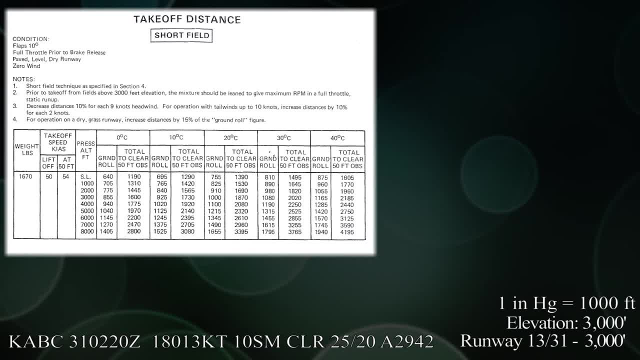 A quick rule of thumb is that 1 inch of mercury equals 1000 feet. So if you take your 2942 and you subtract your altimeter- Yes, do it in that order- Take your altimeter minus 2992.. You'll end up with minus 0.5.. 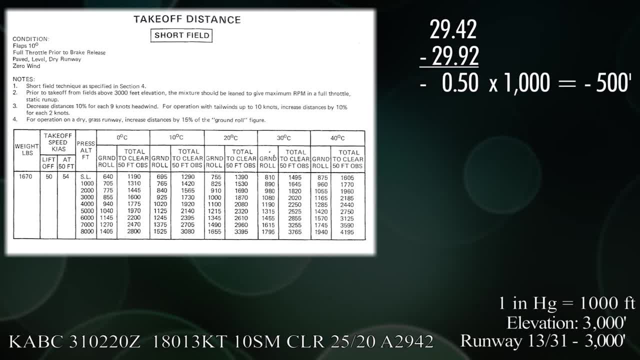 And if you multiply that by 1000. You have minus 500 feet. In other words, you have to take your elevation and subtract 500 feet from it And voila, look at that, You have your pressure altitude of 2500 feet. 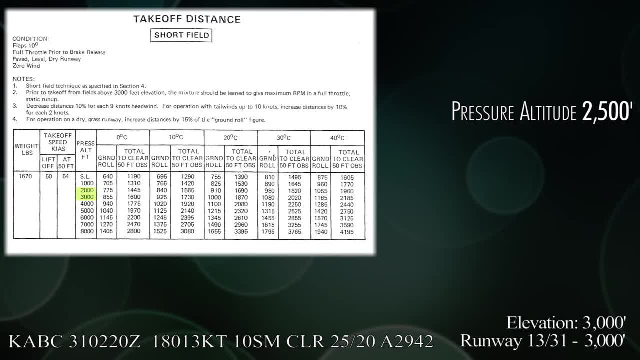 If you look at your chart, there are absolutely no numbers for 2500 feet. If you look at your temperature, There is no temperature for 25 degrees celsius either, Which means you'll have to do a little bit of thinking and some math. 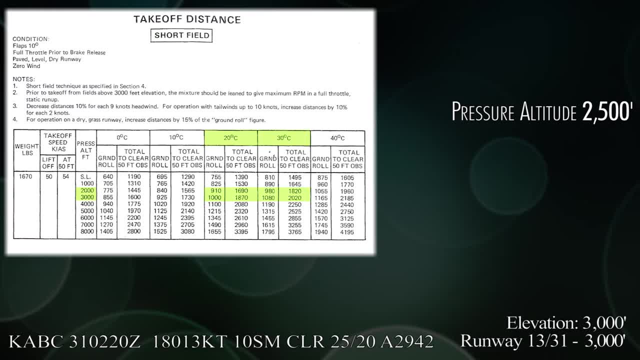 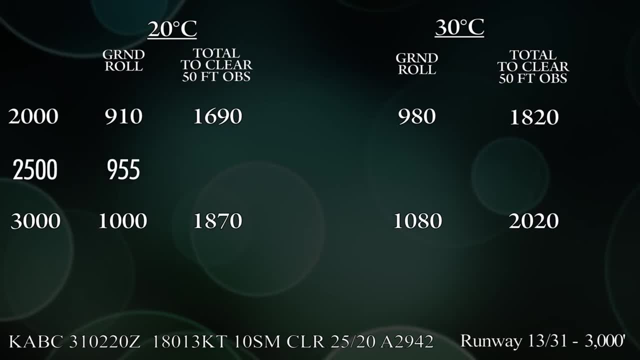 And you'll probably see something like this on the written test, If not for your private, then some point in the future- To get your number. you do a little bit of math And there we go. Look at that, For the ground roll at 2500 feet. 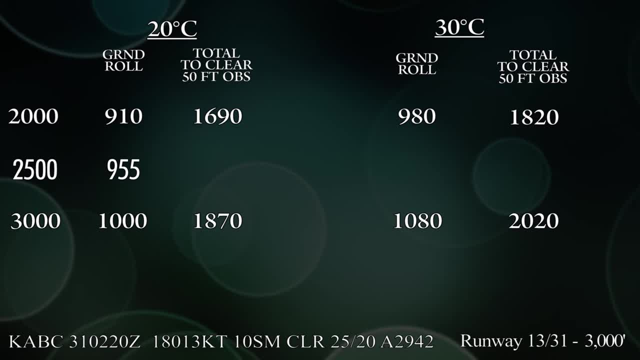 You have 955.. And for the 50 foot obstacle you have 1780.. Then for 30 degrees you have 1030. And then you also have 1920.. So now we have our numbers for 2500 feet. We just don't have them for 25 degrees celsius. 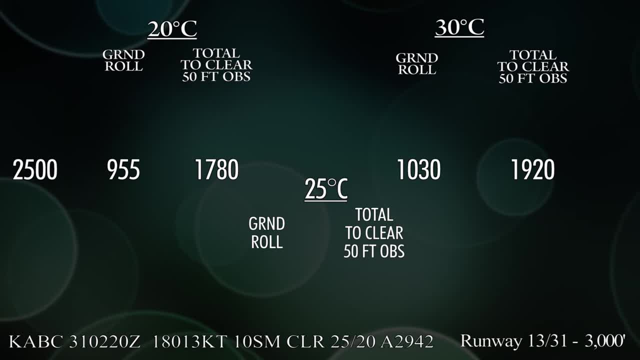 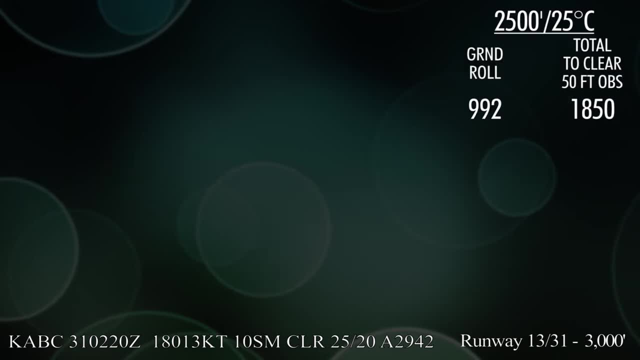 So we'll go ahead and interpolate for that as well, And you get 992 for the ground roll And 1850 for your total to clear a 50 foot obstacle. Alright, so far, so good. Now if we look at note number 3.. 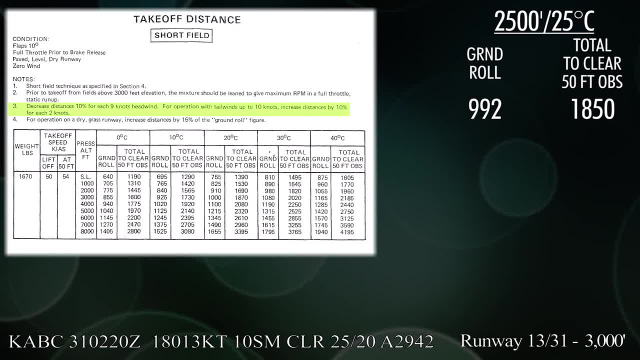 It says: decrease by 10% for every 9 knots again, And so now we come to a little bit of a dilemma. Our wind is 180 and our takeoff runway is 13, or a heading of 130.. That's not an exact headwind. 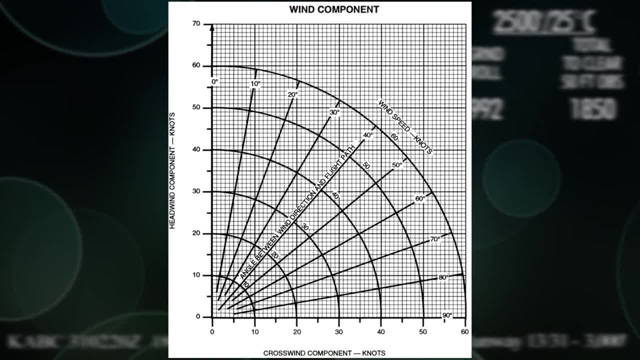 So how do you find your headwind With this lovely chart? On the left side you have headwind. On the bottom you have crosswind. The numbers on each axis: they represent the wind speed. On the outside arc you have degree numbers. 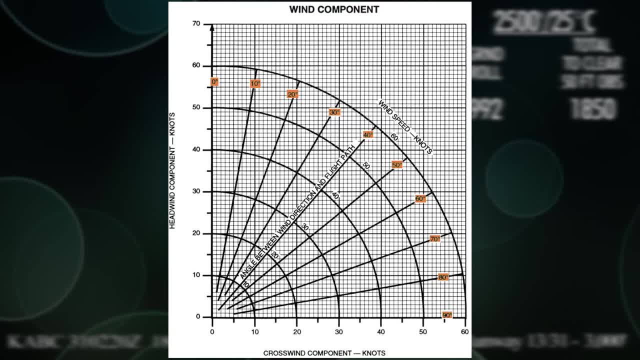 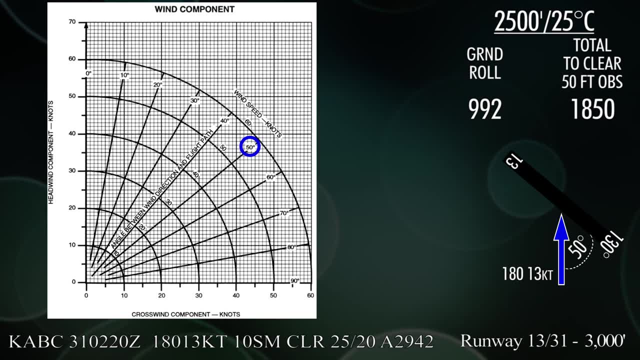 And those are the number of degrees between your runway heading and the wind direction. So in our case we have a 50 degree heading. We have a 50 degree difference between 130 and 180.. So we find 50 on the chart. 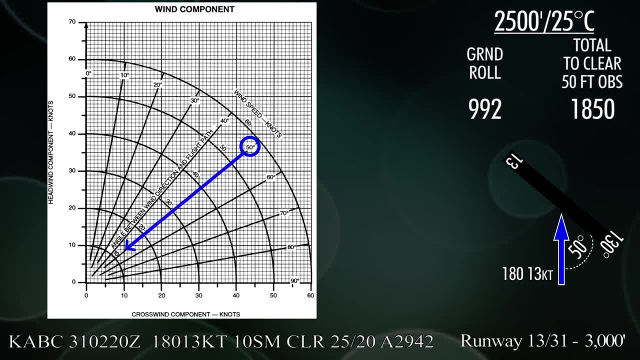 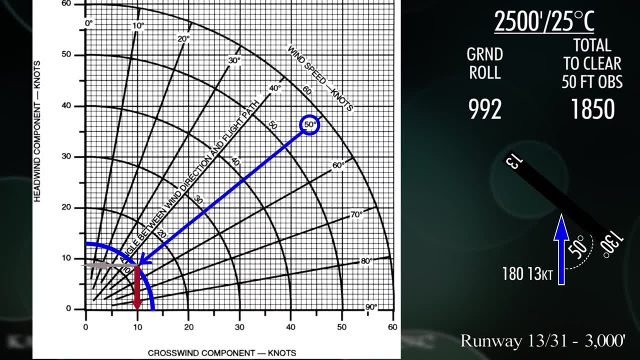 50 degrees difference And then we can follow it down to our wind speed of 13 knots. And if you look straight across to the left, Your headwind is 9 knots roughly And if you look straight down, your crosswind will be about 10 knots for that takeoff. 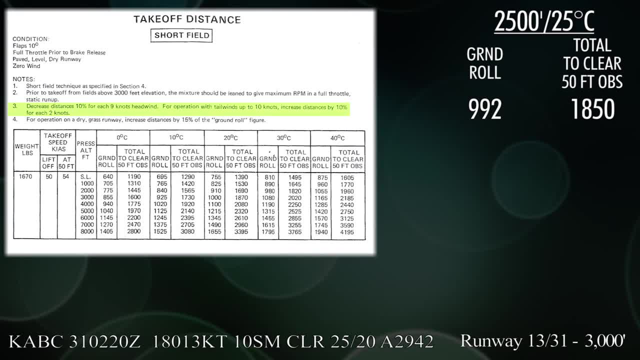 So our headwind is 9 knots. In other words we have to subtract 10% from our takeoff distance once again. So 992 becomes roughly 893. And then 1850 becomes 1665.. Hopefully that made at least a little bit of sense. 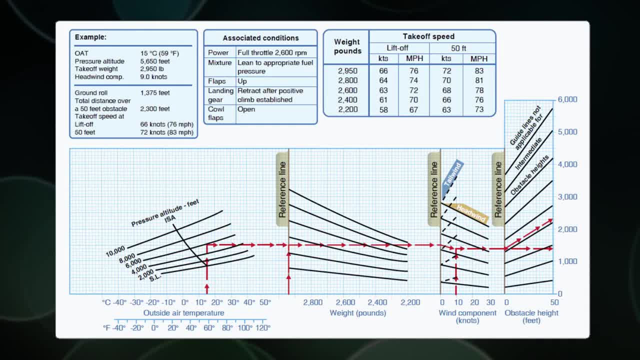 I did go fairly quick through this. Now then onto a different manufacturer's takeoff chart. It looks kind of scary, But it really isn't. Just like with the other chart. there are some conditions And you can read through those if you'd like. 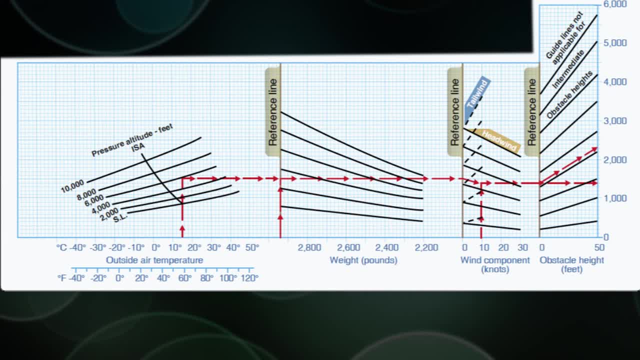 Let's make sure you understand this chart. The way it works is: you follow the pressure altitude line slope Until you meet your temperature, And once those two meet you go straight across. So, for example, if your pressure altitude was 9000. You would follow the slope of those lines for 8 and 10,000. 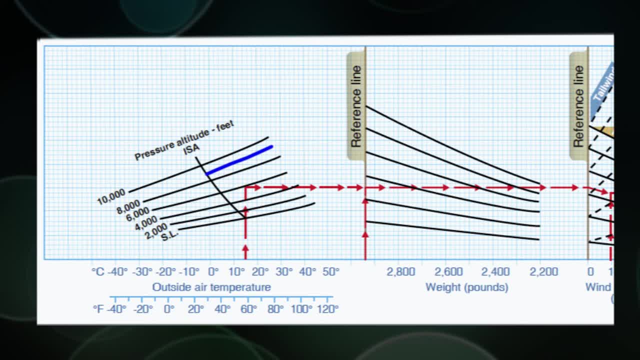 You'd be right in between them And you'd follow that until you met with your temperature. Let's say that your temperature was 20.. So you'd follow the slope of your pressure altitude of 9000 until you met with 20 degrees. 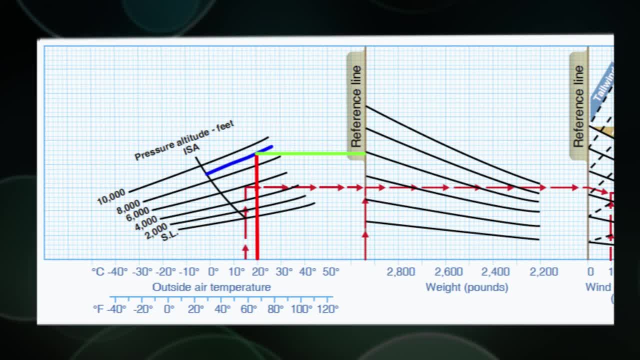 Once those two meet, you can follow straight across to the reference line. Let's do one more, Let's continue on. Let's say that our weight is 2200 pounds, So you would take your line. that's now at the reference line. 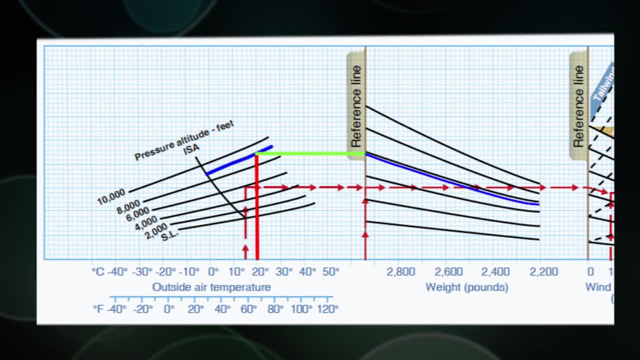 And you would follow the slope of where you ended up All the way down to 2200. And once 2200 and the line that you have meet up, You go straight across to your next reference line. I'm a little bit lazy. 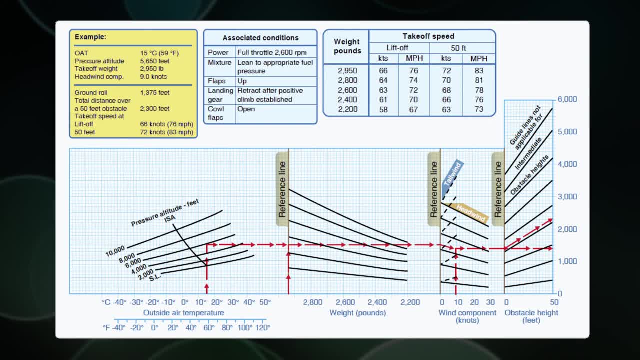 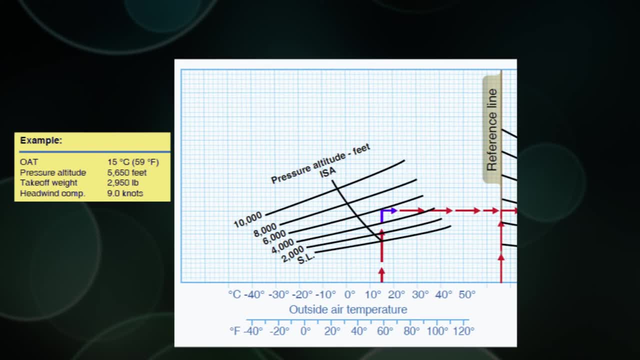 So we'll just follow their example. they have on the left hand side at the top there. So now, looking at this chart, We can follow the temperature on the red line there from the bottom Until it meets our pressure altitude, And our pressure altitude is 5650.. 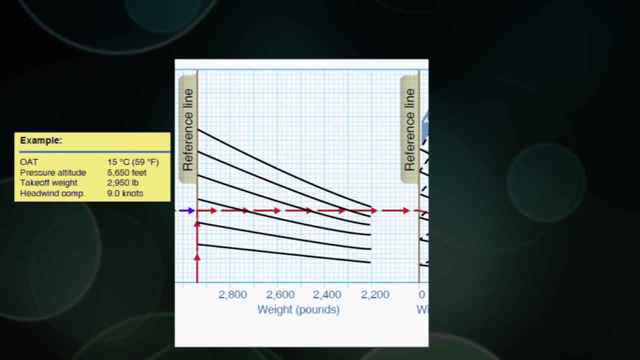 Once those two lines meet, we can run right across over to the next reference line, And that's for weight, And our weight is 2950. Which I'm assuming is the very left hand side. So we don't have to do anything. 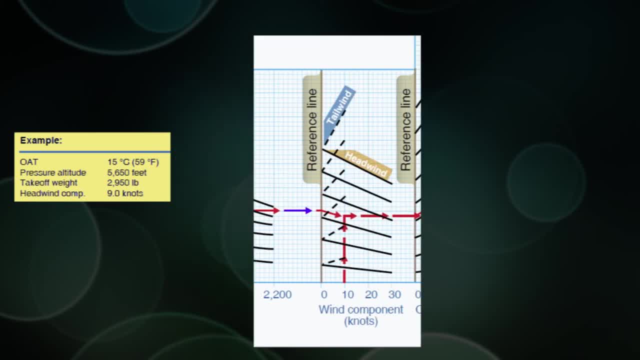 We don't have to follow any sort of lines. We're going right straight across to the next reference line. And then they said we had 9 knots of headwind. For headwind, if you look, you go down, And for tailwind, you would go up. 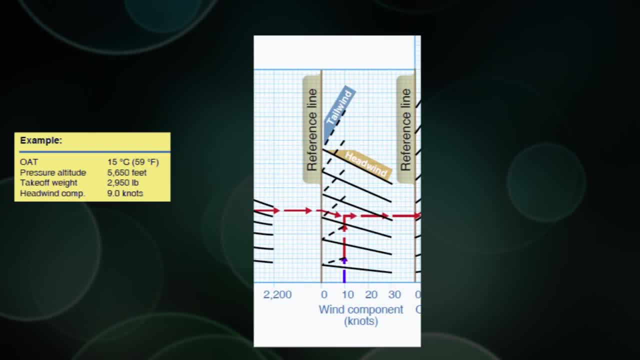 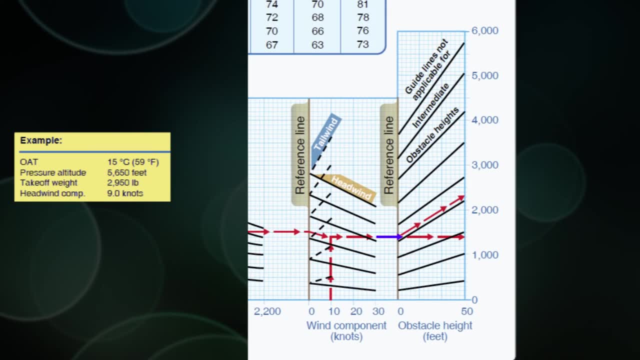 So for 9 knots of headwind We parallel that line and go down to 9 knots And then, once those lines meet, again 9 knots and the line that we have, We go straight across to the next reference line. If we want to know our ground roll, we go straight across. 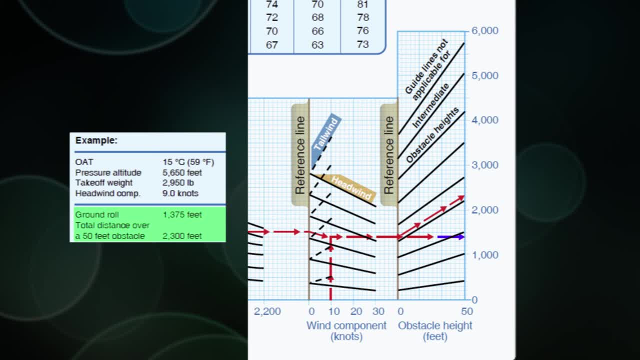 And that's going to be 1375.. And if we want to know our take off over 50 foot obstacle, Then we go follow the slant of the line To the end of the line, or 50 feet, And that happens to be 2300 feet. 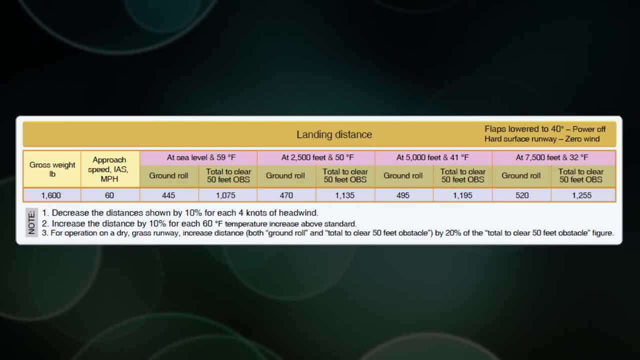 I hope that wasn't super difficult to figure out. Here's another, just in Fahrenheit and not Celsius, And miles per hour instead of knots. Also, this is for landing distance, Which is kind of what we're going to look at next. So for landing distance, 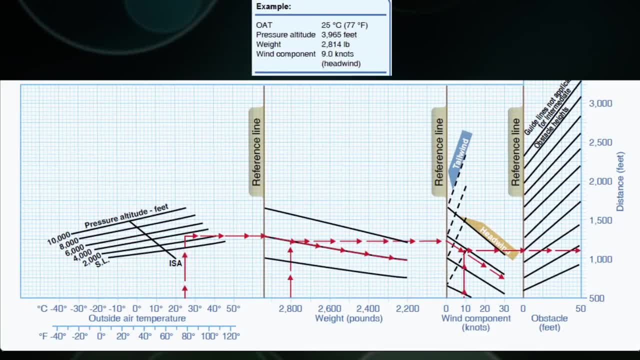 We're going to be doing the same sort of thing You have. let's see what do we have: 25 degrees Celsius Pressure, altitude of, let's say, 4000 feet, Weight of 2800 pounds And 9 knots of headwind. 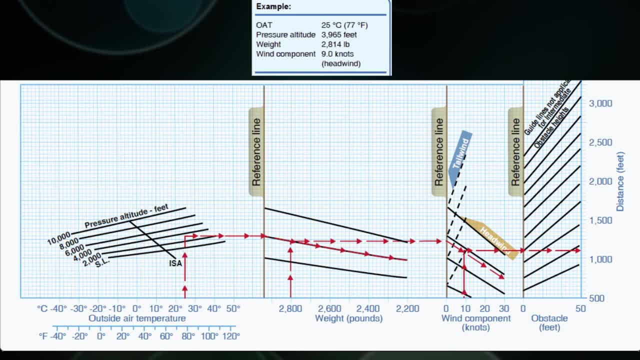 And so we go and follow from 25 degrees Up until we meet roughly 4000 feet of pressure altitude And then jog right across to the reference line And our weight is now 2800 pounds. So we follow the slant of the line to 2800.. 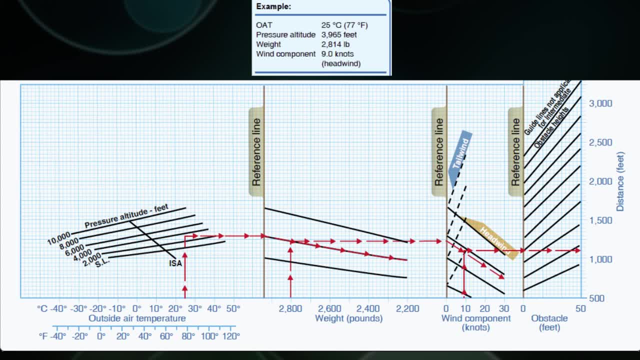 And then go right across all the way to the next reference line. Our headwind is 9 knots, So we'll follow the down sloping line until 9 knots And then go right across to the next line. Our ground roll for the landing distance.